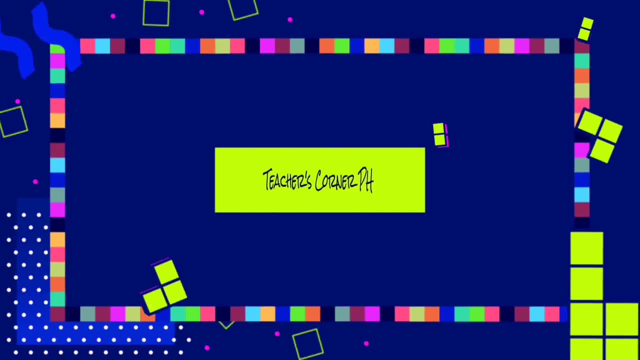 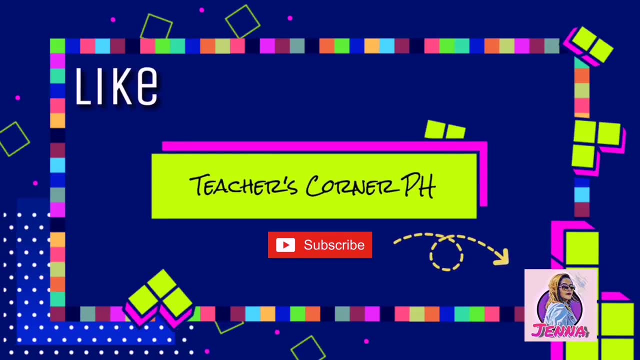 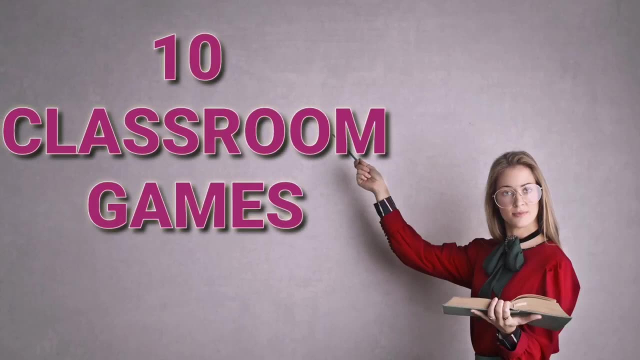 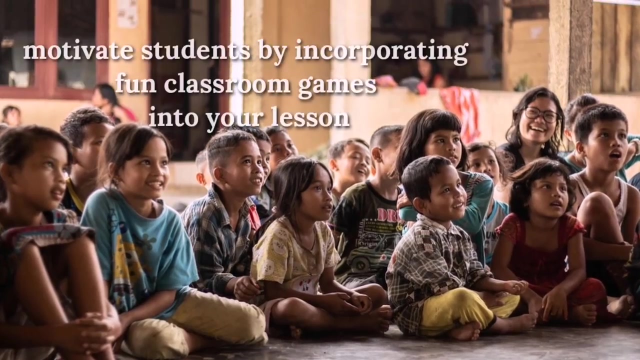 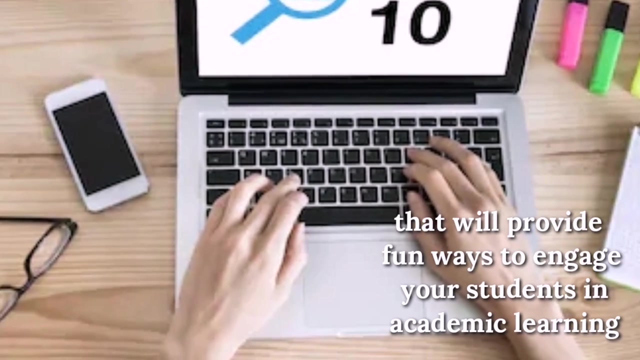 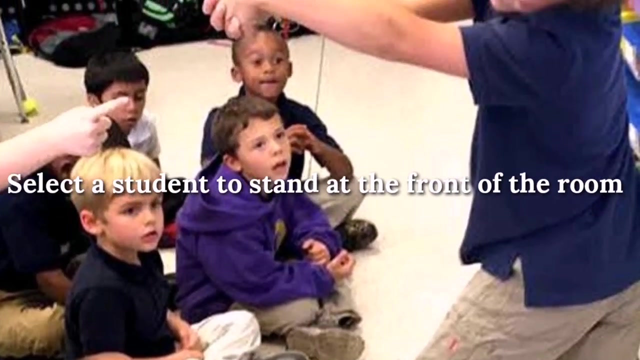 It is important to make learning exciting for students. Motivate students by incorporating fun classroom games into your lesson. Here are the top 10 classroom games that will provide fun ways to engage your students in academic learning. Number 1. Charades: Select a student to stand at the front of the room and 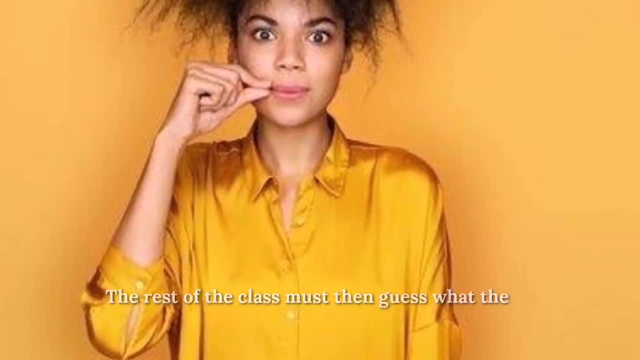 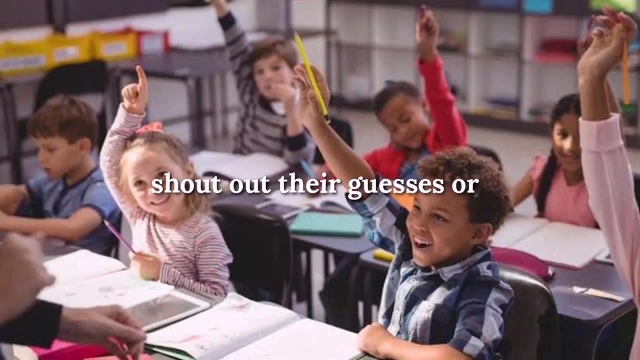 act out a word from your list, No speaking aloud. The rest of the class must then guess what the student is attempting to portray. Other students can shout out their guesses or put their hands up, depending on your teaching preference. Whoever guesses correctly can act out the next word. 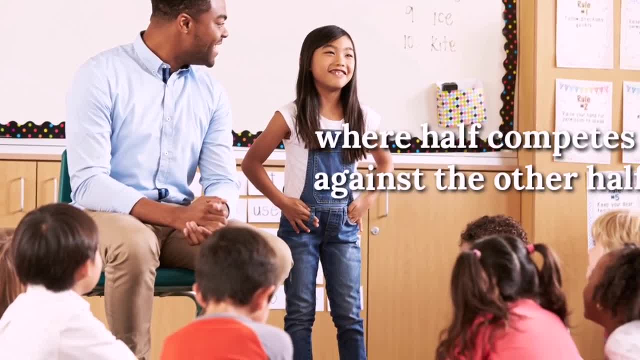 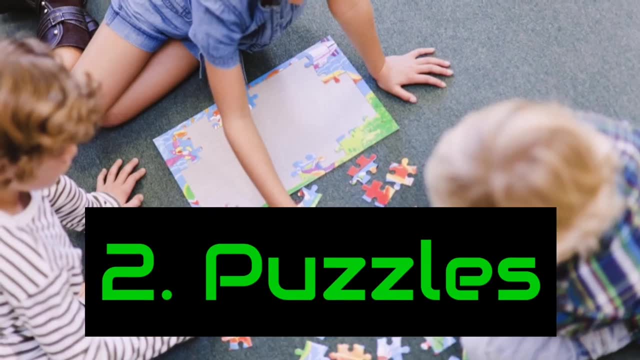 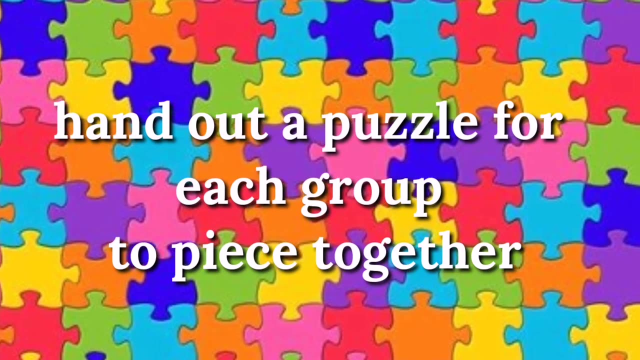 You might like to experiment with playing as a whole class, where half competes against the other half, or in smaller groups with time limits. Number 2. Puzzles. Separate your class into groups or simply use table groupings. Then hand out a puzzle for each group to piece together. You may use 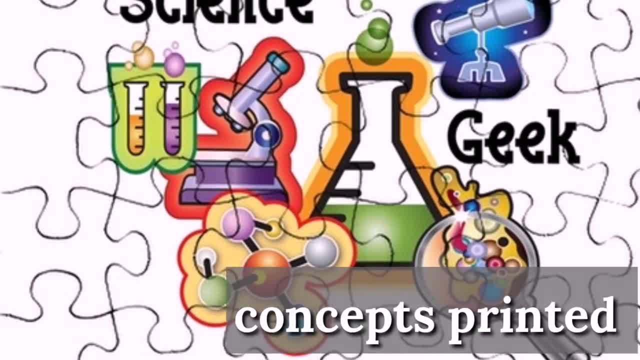 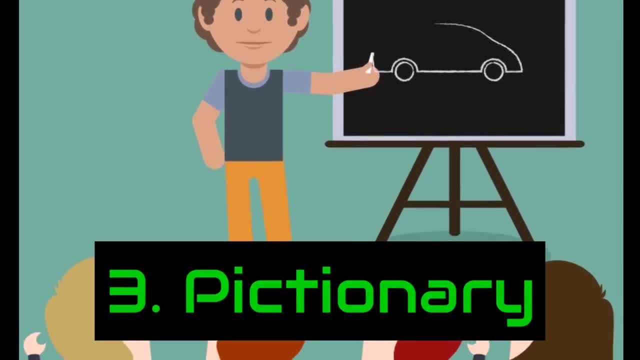 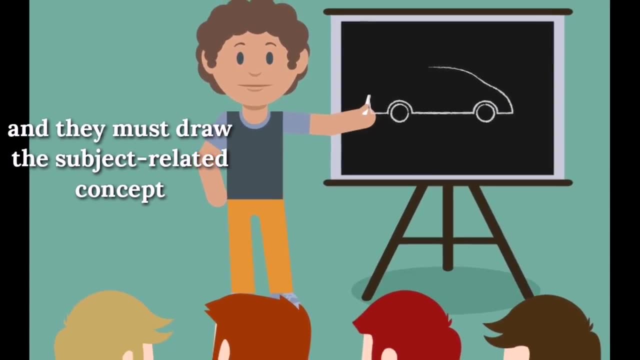 images, words, calculations or concepts printed or stuck on card or paper and cut into random shapes like puzzle pieces. Number 3. Pictionary Students work in small groups. One student from each group is chosen to start and they must draw the subject-related concept you state. 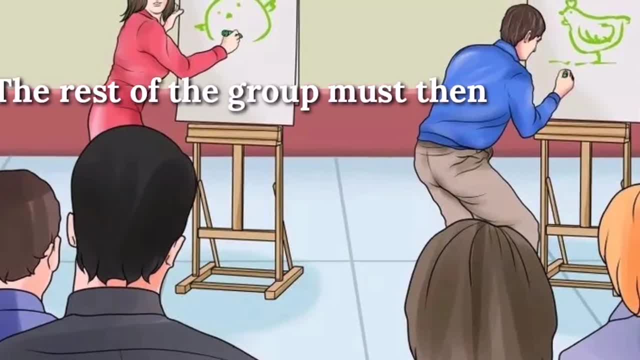 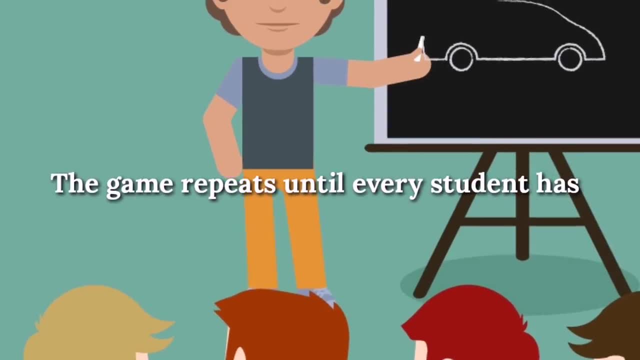 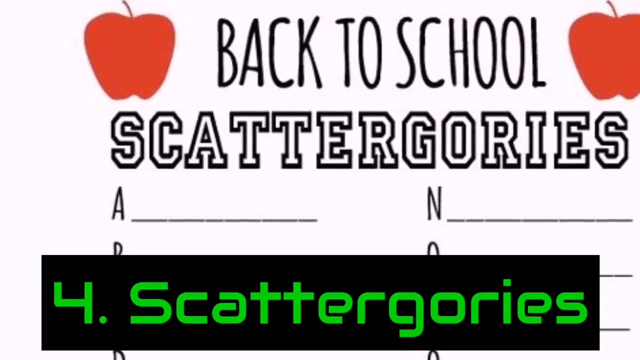 within a given time- 30 seconds to 2 minutes. The rest of the group must then guess what she is drawing. The first group to correctly guess the word wins. The game repeats until every student has had a turn or there are no more words on your list, Number 4. Scattergories. 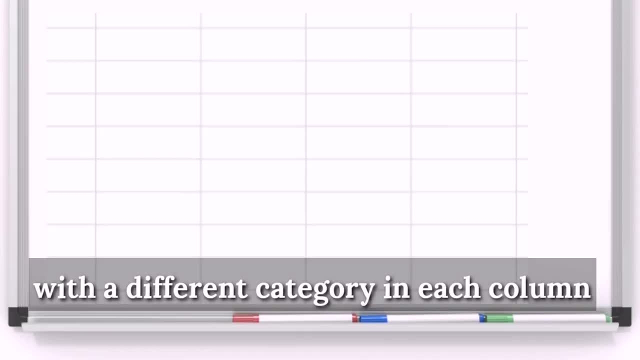 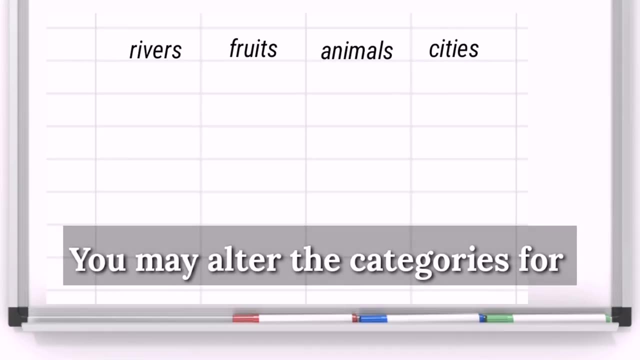 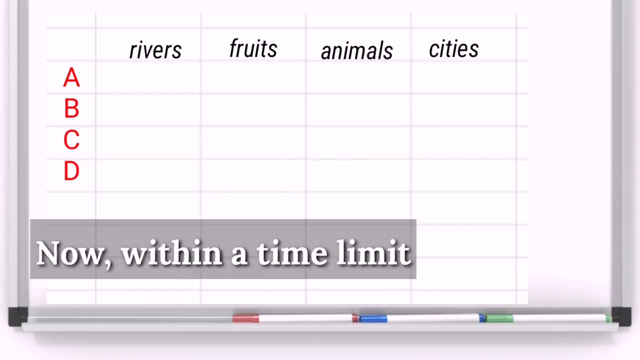 Put up a simple table on the whiteboard with a different category in each column, For example, rivers, fruits, animals or cities. You may alter the categories for difficulty according to your class's level. Randomly select a letter of the alphabet Now, within a time limit, groups or. 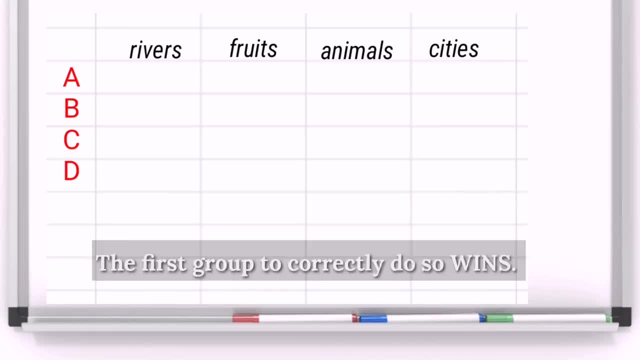 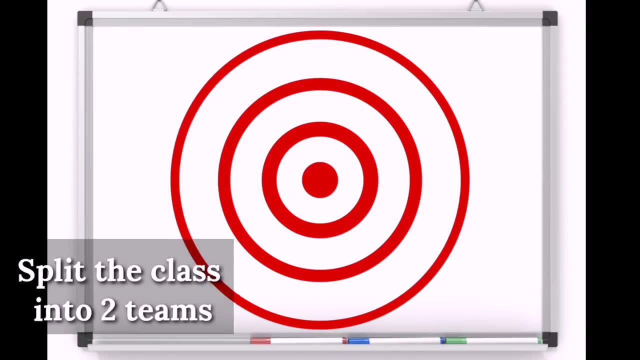 pairs of students must identify one example per category. The first group to correctly do so wins Number 5. Whiteboard Bullseye. Split the class into two teams. Draw a target on the whiteboard Labeling each circular ring with a different point value. Quiz students individually on anything you want, If they. 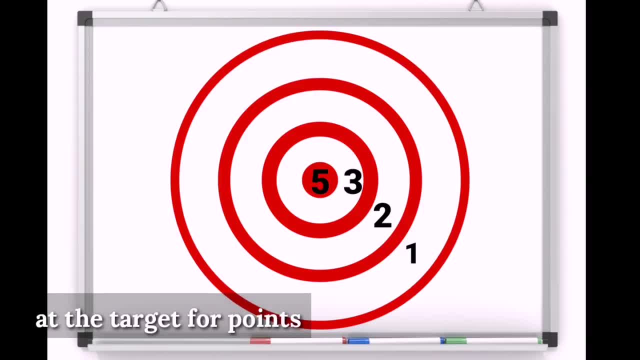 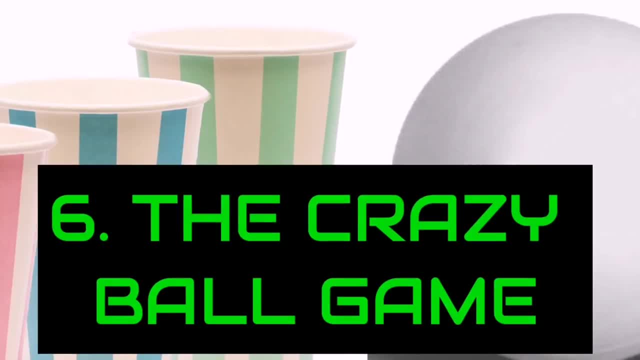 answer correctly, they get to throw the ball at the target for points. The winning team gets a prize, a bonus point on the test, a privilege, etc. Number 6. The Crazy Ball Game. Prepare a questionnaire for the game based on a topic that you taught recently to the class. 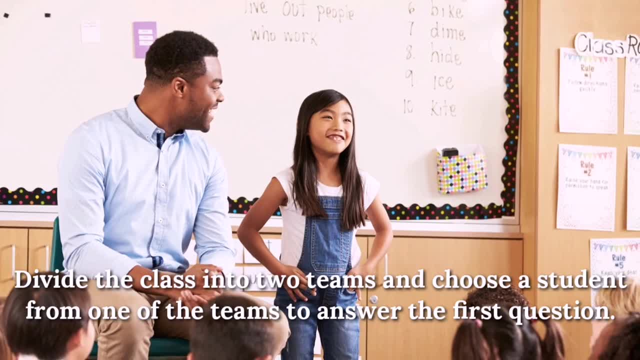 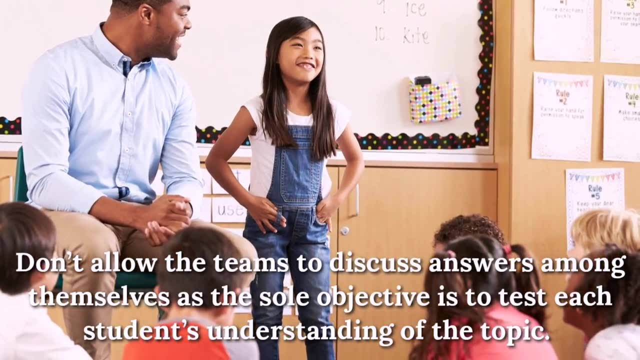 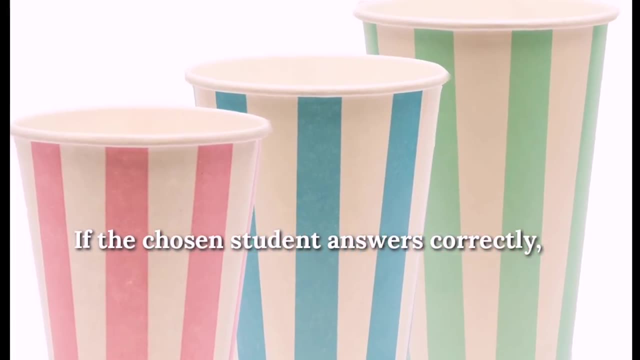 Divide the class into two teams And choose a student from one of the teams to answer the first question. Don't allow the teams to discuss answers among themselves, as the sole objective is to test each student's understanding of the topic. If the chosen student answers correctly, she gets to throw a ball into one. 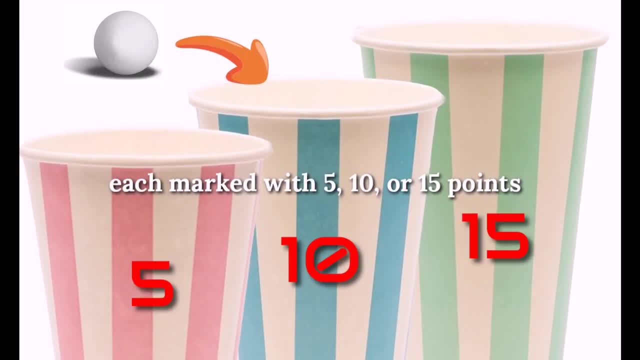 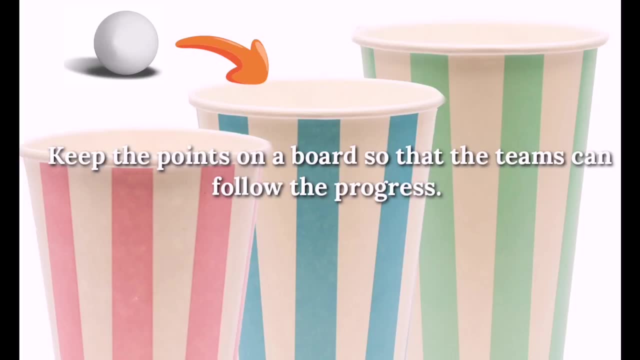 of three paper cups, each marked with 5,, 10, or 15 points, and get points for her team. Keep the points on a board so that the teams can follow the progress. Continue to play the game between the teams until you've asked all the questions. 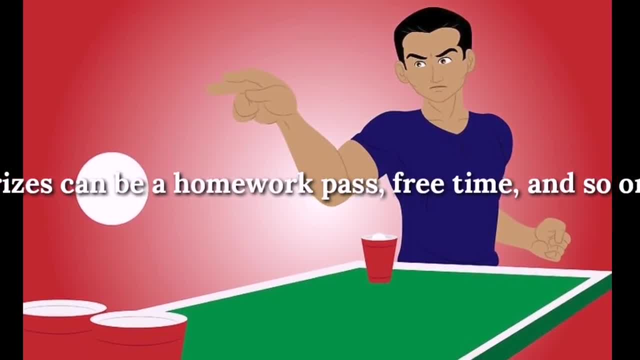 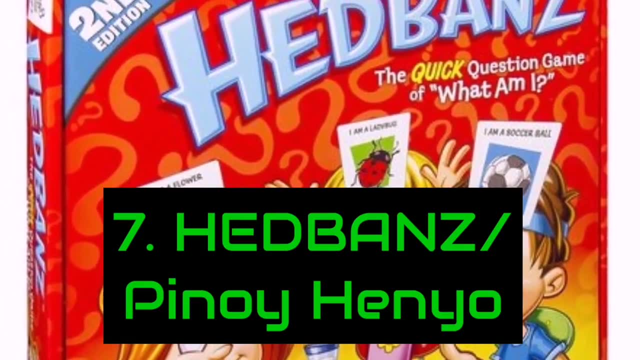 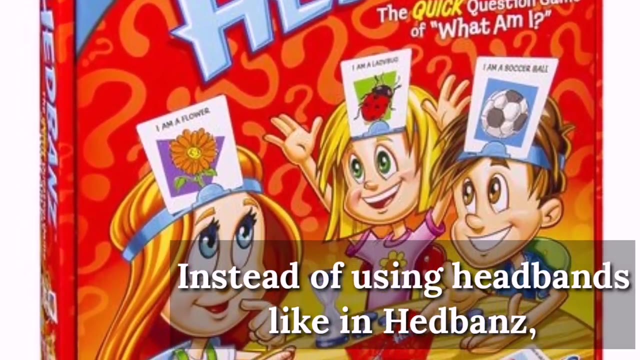 The team with the maximum number of points wins. Prizes can be a homework, pass free time and so on. Number 7.. Headbands are also known as Pinoy Henyo. Here's a fun spin on the classic game of headbands. Instead of using headbands like in headbands. 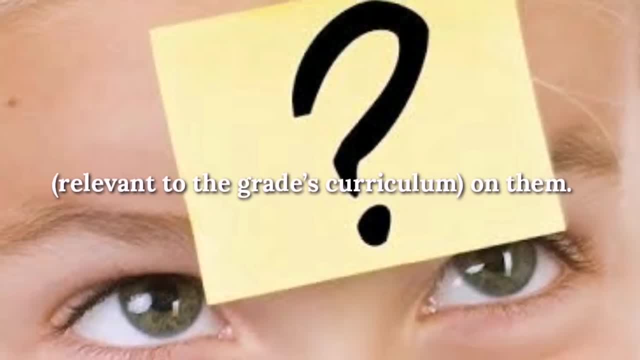 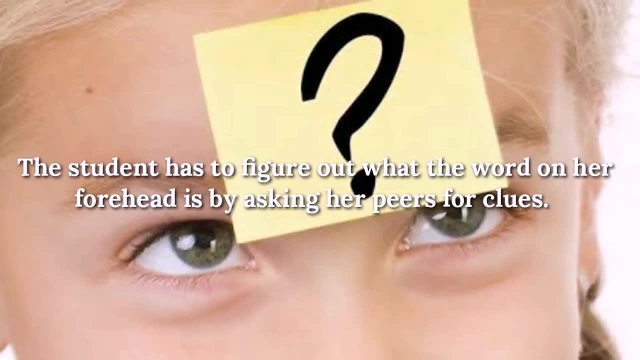 use sticky notes to write random words relevant to the grade's curriculum on them. Stick one of the notes on a student's head without allowing her to look at the word. The student has to figure out what the word on her forehead is by asking her peers for clues. 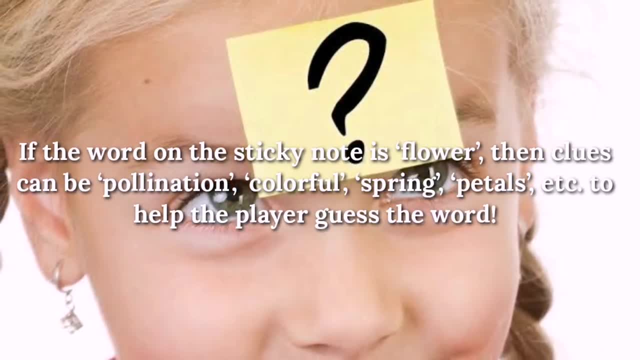 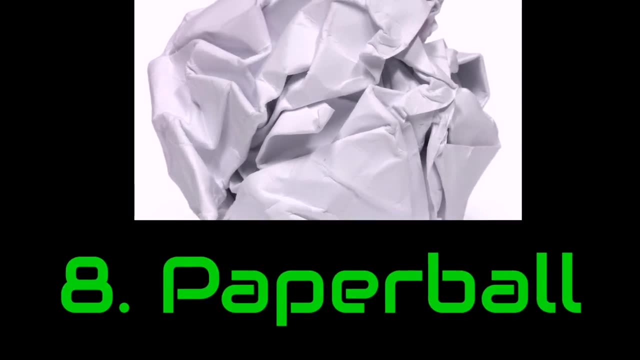 If the word on the sticky note is flower, then clues can be pollination, colorful spring petals, etc. to help the player guess the word Number 8.. Paper ball. Get a piece of paper and write a question on it. 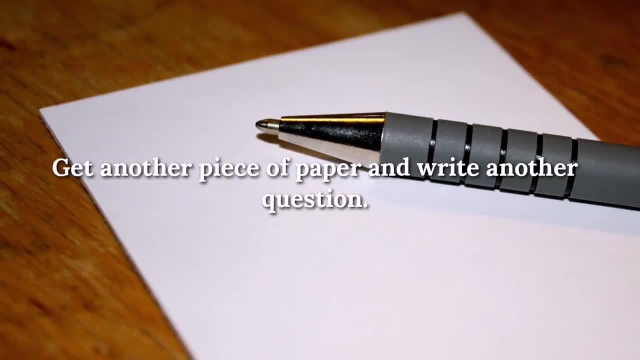 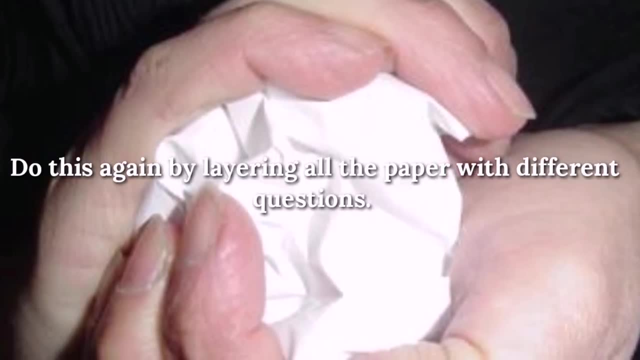 Crumple the paper. Get another piece of paper and write another question. Crumple the second paper by layering it on the first crumpled paper. Do this again by layering all the paper with different questions. You now have a paper ball. Have the students sit in a circle. 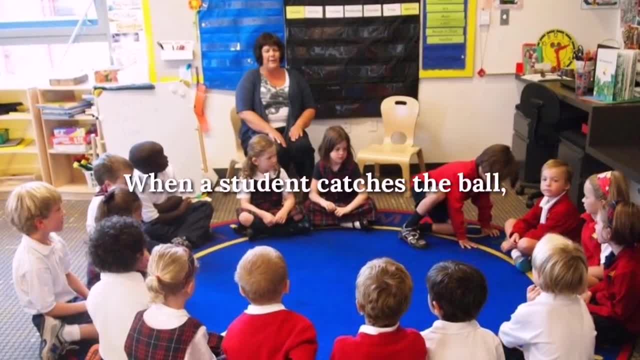 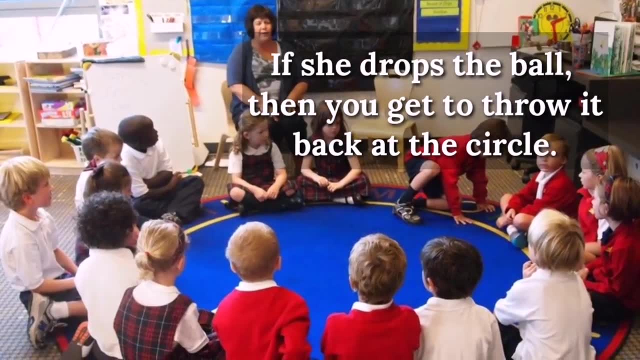 The objective of the game is to play, catch or pass the paper ball. When a student catches the ball, she has to answer the question written on the first layer of the paper ball. If she drops the ball, then you get to throw it back at the circle.